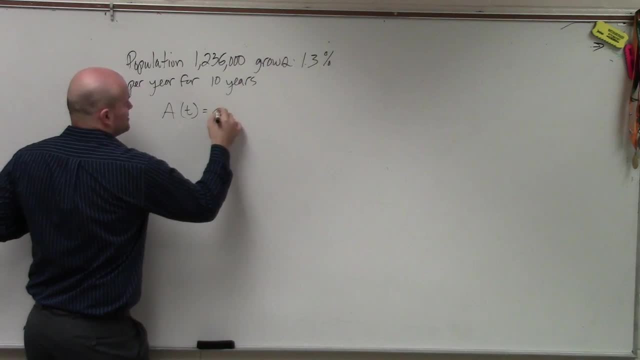 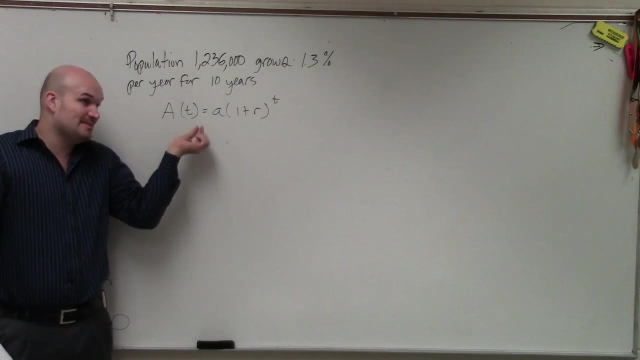 and then we talked about the modeling function, which would be: a of t equals a times 1 plus r raised to the t right. So remember, a of t was the amount after t periods. a was your initial amount, r was your rate and t was your number of time periods. 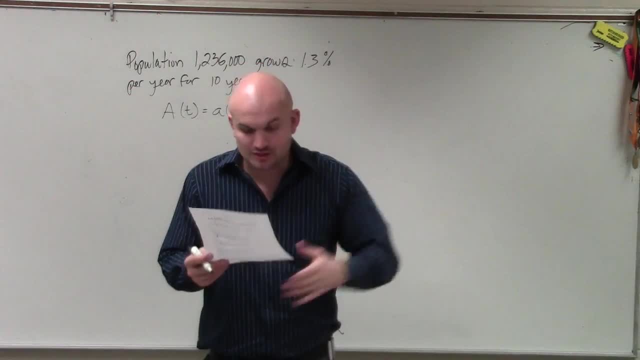 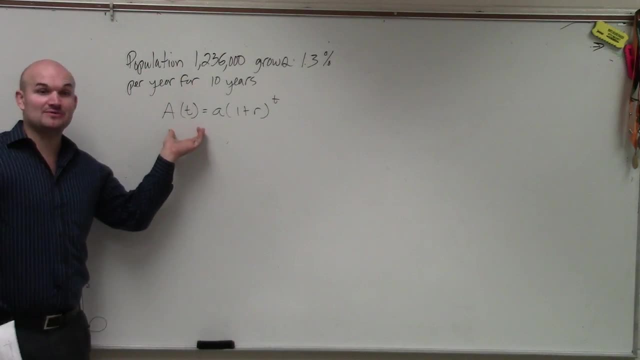 So the question- remember, I told you guys about restating the question. The question is saying: find the amount after the specified time. So are we looking for a of t, which is the amount after the time? Yeah, it's the same. 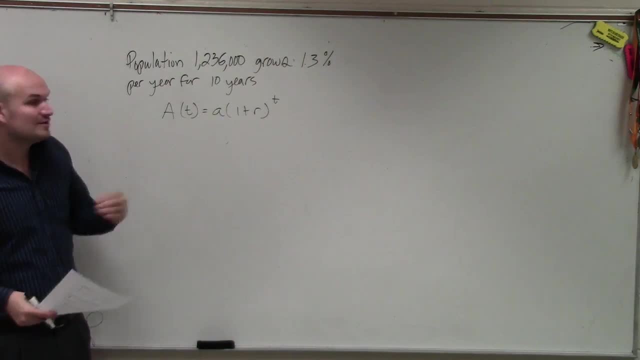 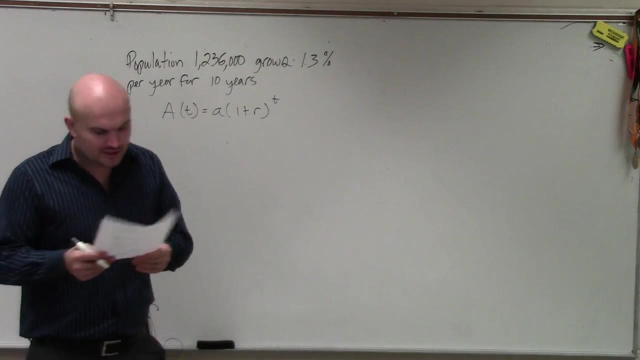 That just restated it right. So yeah, we're looking for a of t. So that means I need to find a value for a, I need to find a value for r and I need to find a value for t. So I go looking into the problem and it says a population of 1,236,000 grows. 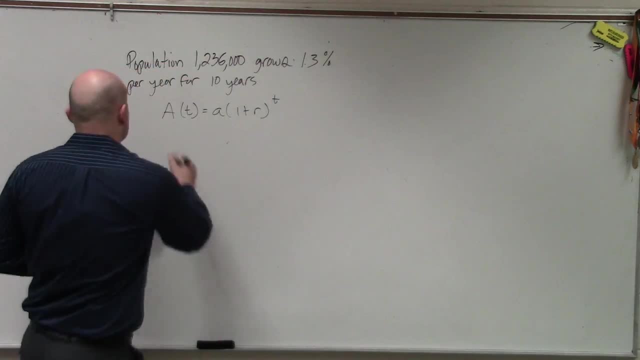 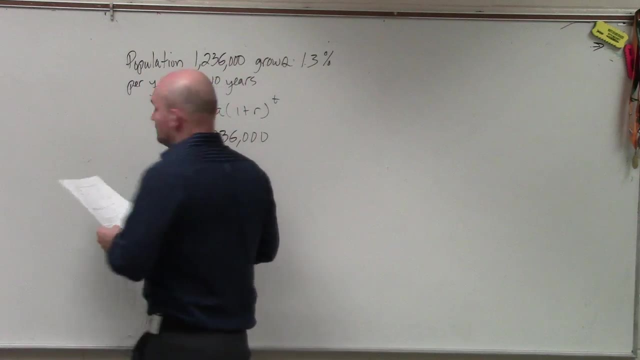 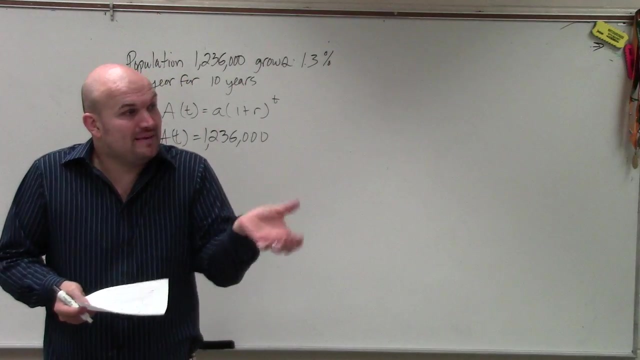 So therefore, I could say that the initial population is going to be 1,236,000.. Would everybody agree? Now it says it's growing, right? So if it's going to grow, then therefore I know that my b, my eventual b, is going to be greater than 1.. 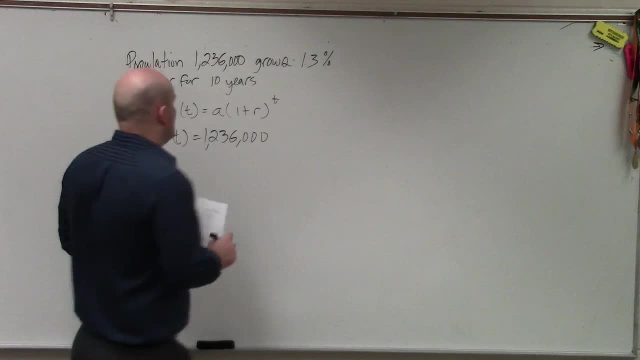 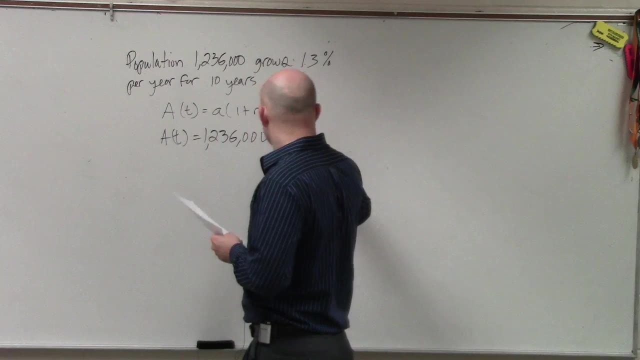 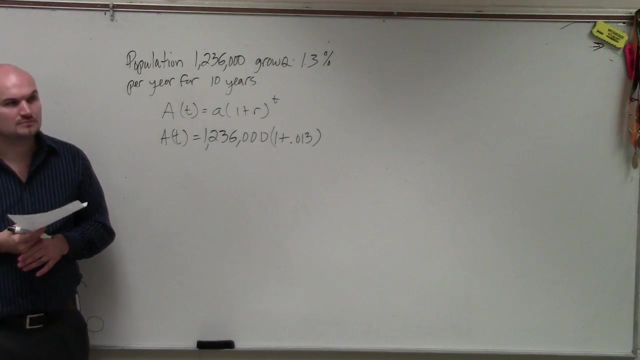 Would everybody agree with me, Right? Because, remember, b had to be greater than 1.. So my interest rate, though remember we always represented interest rate in decimal form, So that's going to be 1 plus .013.. Does everybody agree with me on that? 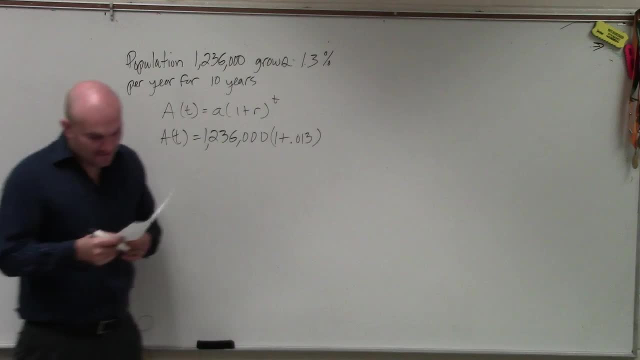 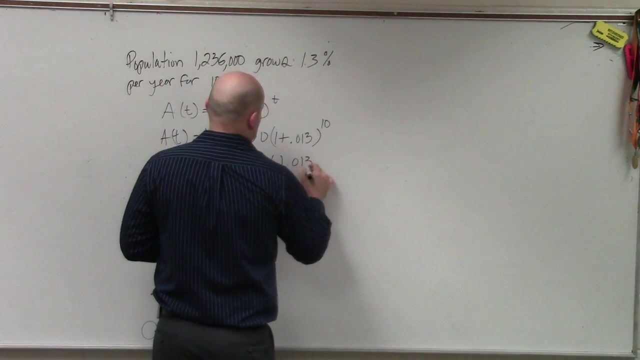 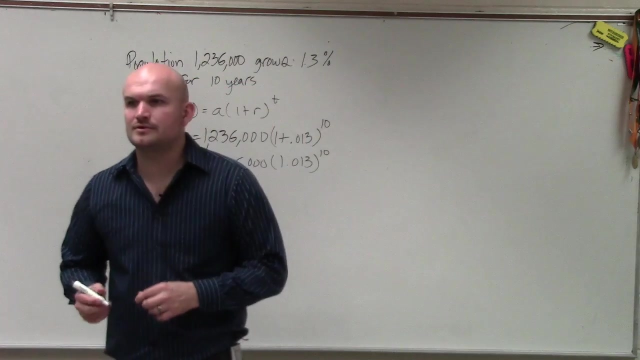 Decimal form of 1%, 1.3%. Okay, And then the t- Our time period is going to be 10 years, So I can just simplify inside my parentheses. Okay, And then I just take my calculator. Who stole my calculator? 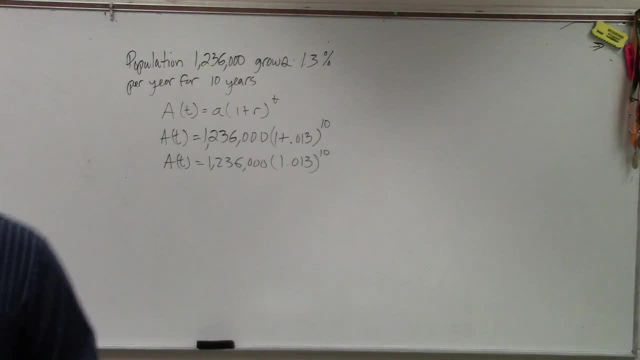 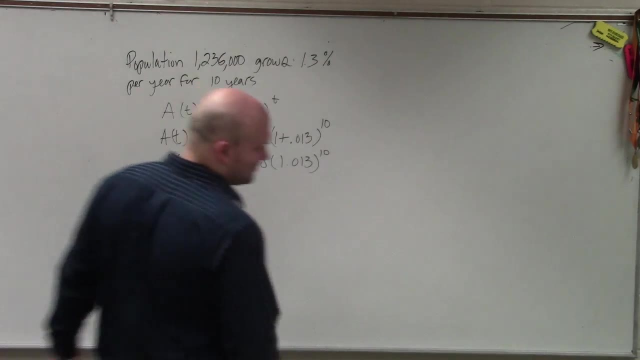 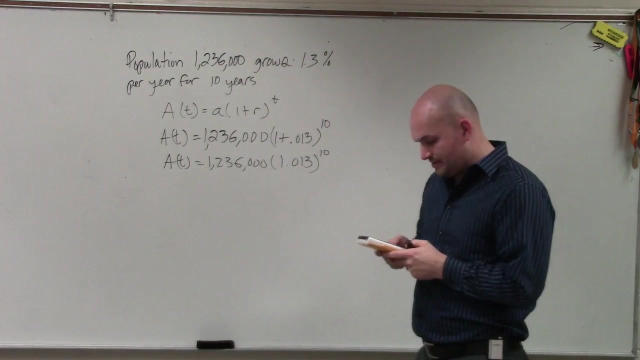 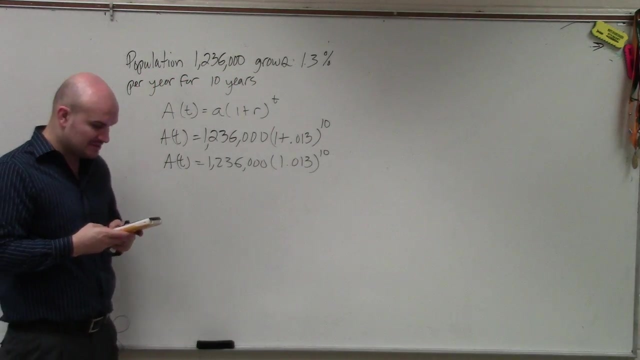 Who stole my calculator? Huh, Ah, I see what you guys are trying to do. You're trying to hide my calculator from me, Thank you. So I'll do 1.013 raised to the 10th power, And then I'm going to multiply that by 1,236,000.